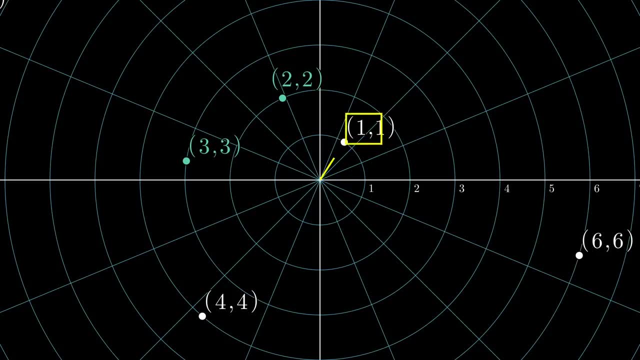 the primes. The point sits a distance 1 away from the origin, with an angle of 1 radian, which actually means this arc is the same length as that radius, And then 2,2 has twice that angle and twice the distance. 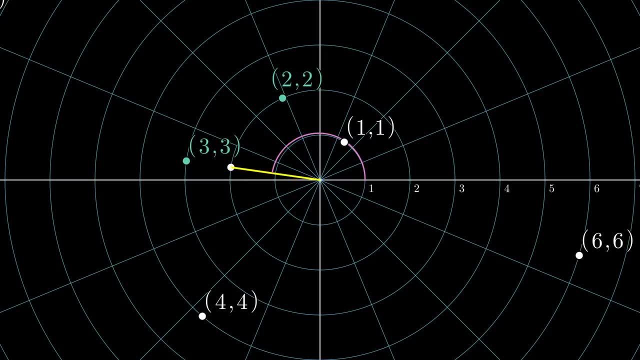 And to get to 3,3, you rotate one more radian with a total angle that's now slightly less than a half turn, since 3 is slightly less than pi, and you step one unit farther away from the origin. I really want you to make sure that it's clear what's being plotted, because everything 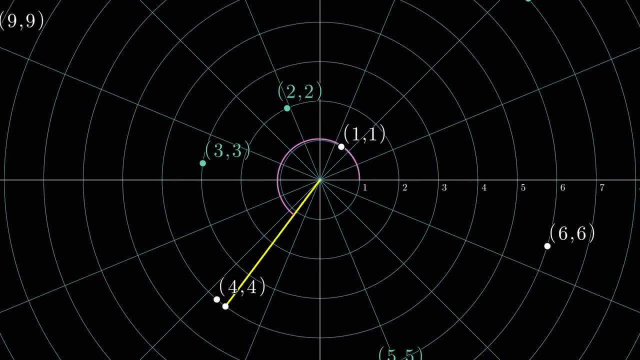 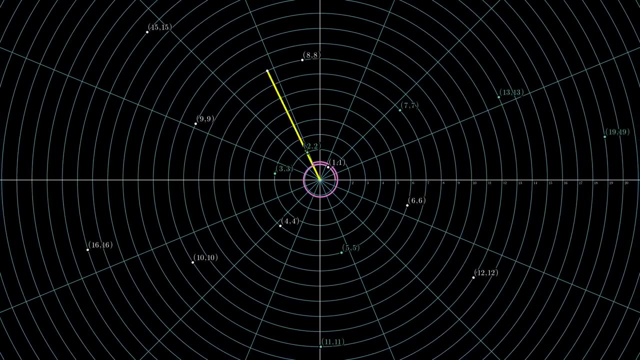 that follows depends on understanding it. Each step forward is like the tip of a clock hand, which rotates one radian. with each tick, a little less than a sixth of a turn, And it grows by one unit. As you continue, these points spiral outwards, forming what's known in the business as 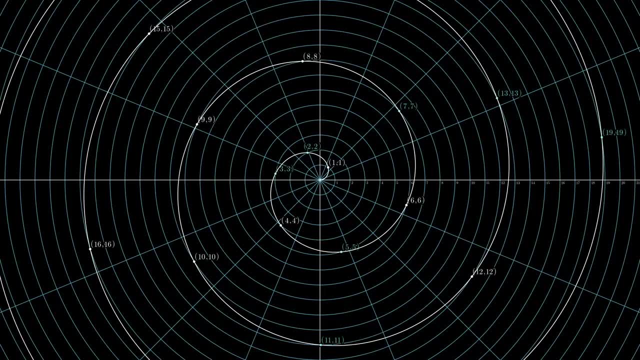 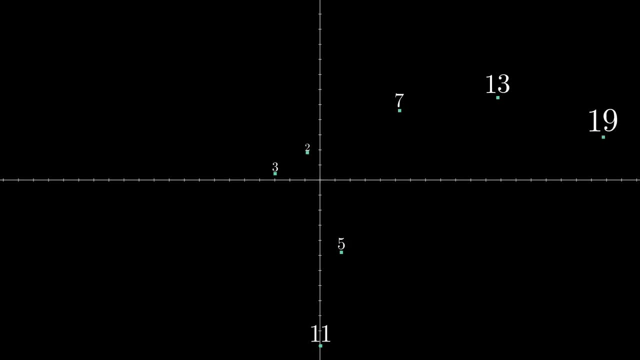 an Archimedean spiral. Now, if you make the- admittedly arbitrary- move to knock out everything except the prime numbers, it initially looks quite random. After all, primes are famous for their chaotic and difficult-to-predict behavior. But when you zoom out, what you start to see are these very clear galactic-seeming spirals. 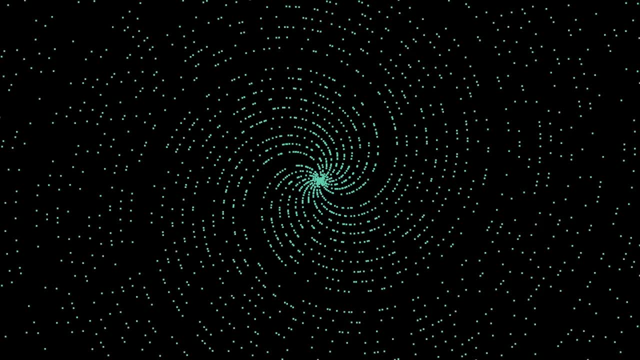 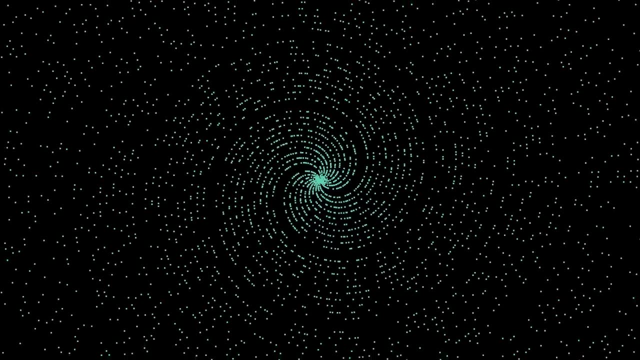 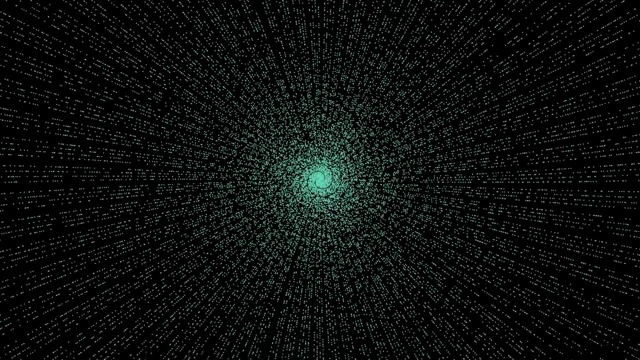 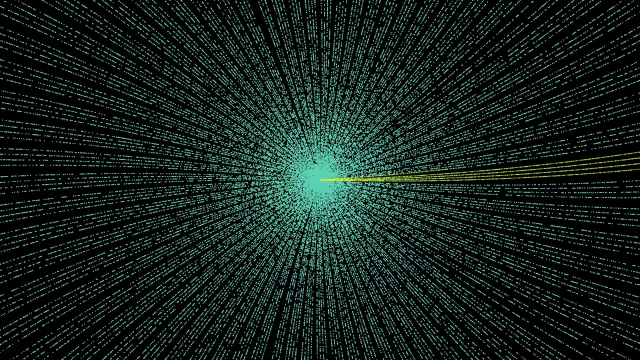 And what's weird is that some of the arms seem to be missing And zooming out even further. those spirals give way to a different pattern, These many different outward-pointing rays, And those rays seem to mostly come in clumps of four, but there's the occasional gap, like a comb missing its teeth, And those rays seem to mostly come in clumps of four, but there's the occasional gap like a comb missing its teeth, And those rays seem to mostly come in clumps of four, but there's the occasional gap, like a comb missing its teeth. 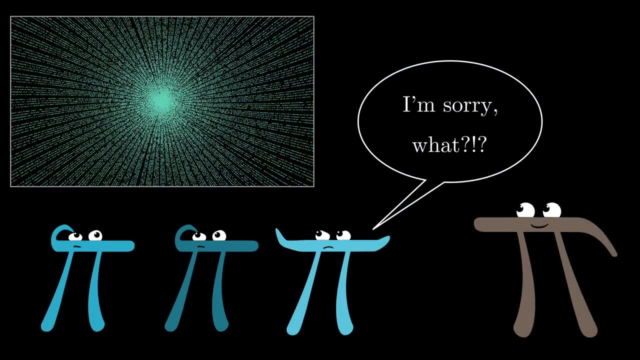 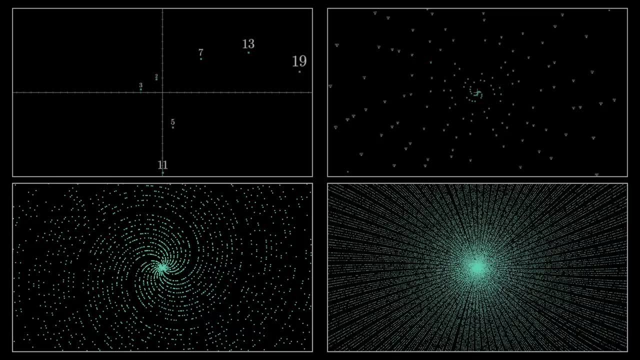 The question for you and me, naturally, is what on earth is going on here, Where do these spirals come from, And why do we instead get straight lines at this larger scale? If you wanted, you could ask a more quantitative question and count that there are 20 total. 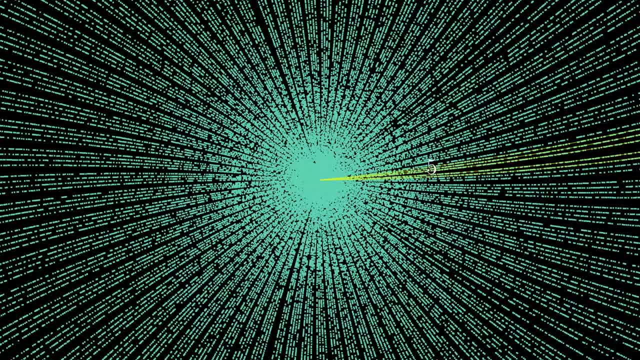 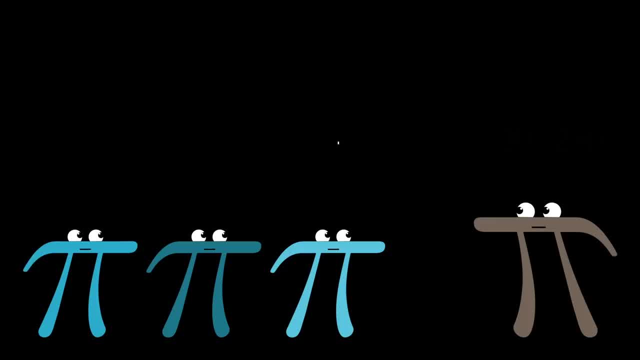 spirals, And then up at that larger scale. if you patiently went through each ray, you'd count up a total of 280. And so this adds a further mystery of where these numbers are coming from and why they would arise from primes. 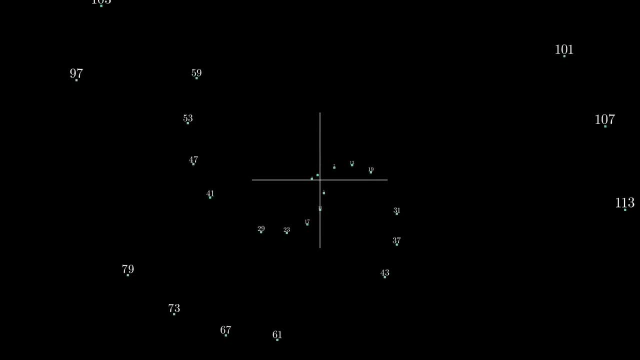 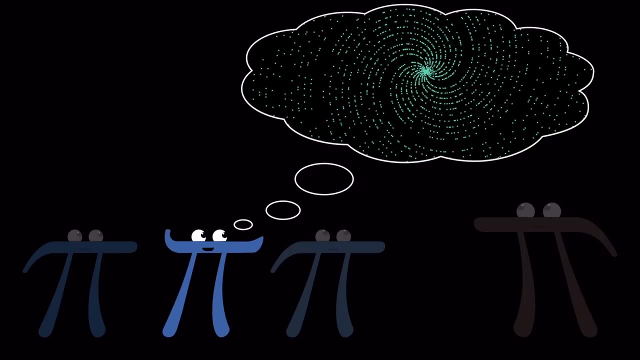 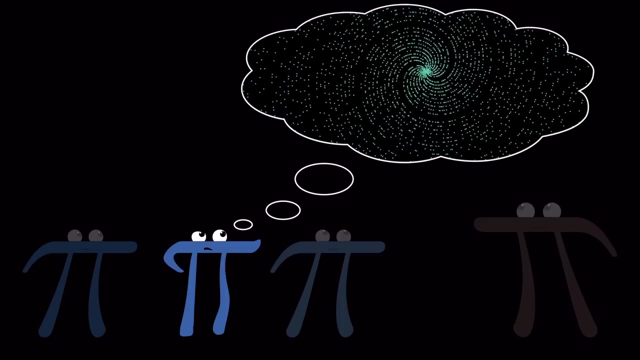 Now, this is shocking and beautiful, and you might think that it suggests some divine hidden symmetry within the primes. But to steady your expectations, I should say that the fact that the person asking this question on math exchange jumped right into prime numbers makes the puzzle a little misleading. 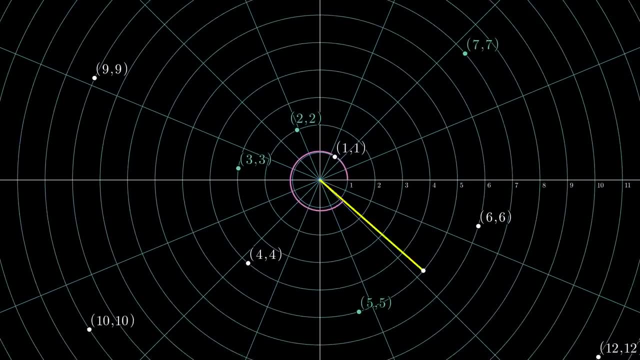 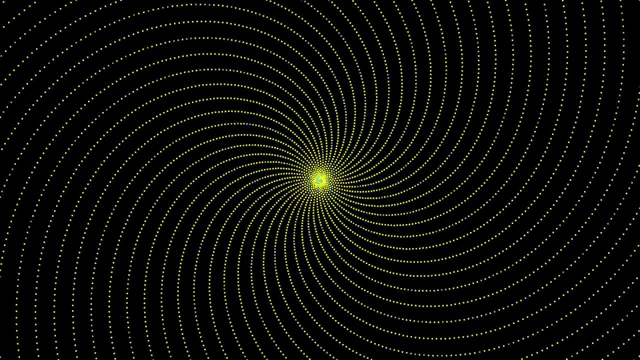 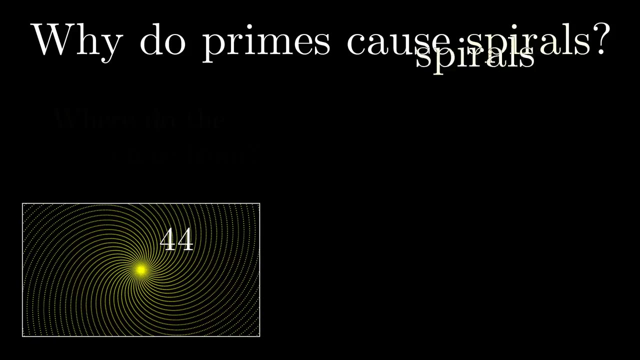 If you look at all of the whole numbers, not just the primes, as you zoom out, you see very similar spirals. They're much closer, They're much cleaner And now there's 44 of them instead of 20.. But it means that the question of where the spirals come from is perhaps disappointingly. 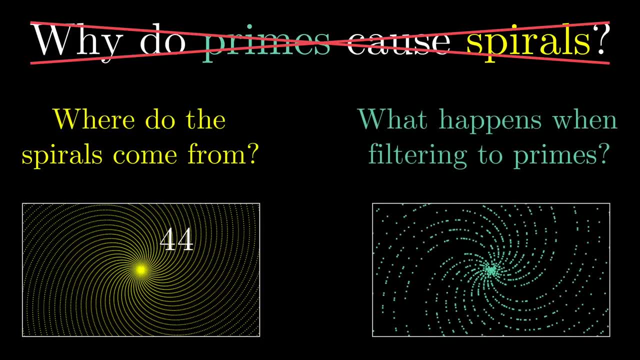 completely separate from the question of what happens when we limit our view to primes. But don't be too disappointed, because both these questions are still phenomenal puzzles. There's a very satisfying answer for the spirals and even if the primes don't cause. 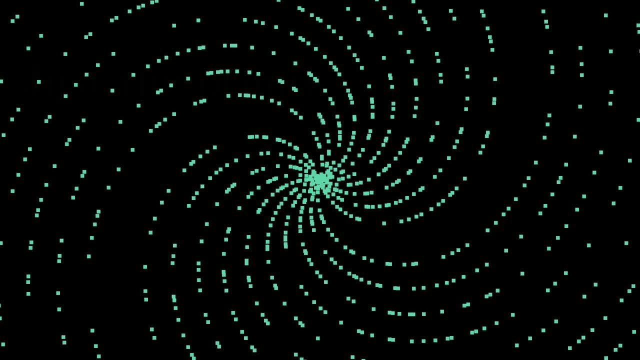 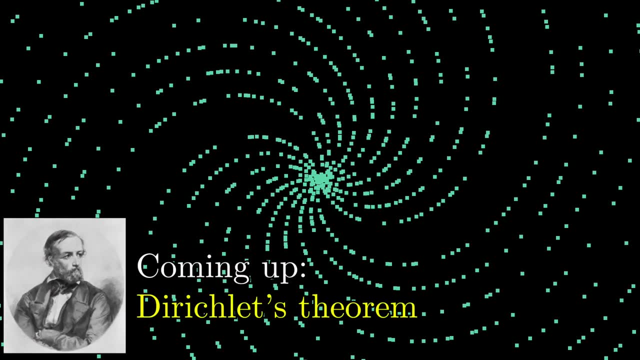 the spirals. asking what goes on when you filter for those primes does lead you to one of the most important theorems about the distribution of prime numbers: The question of what happens when we limit our view to primes. This is known in number theory as Dirichlet's theorem. 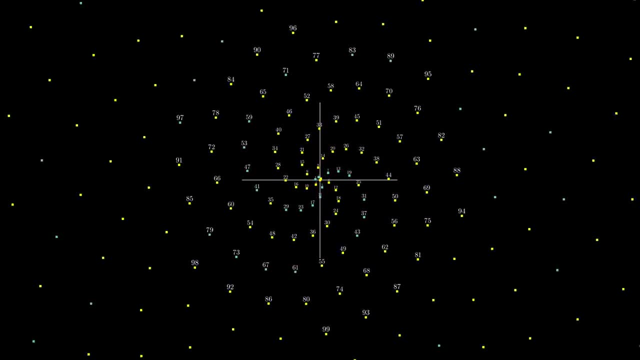 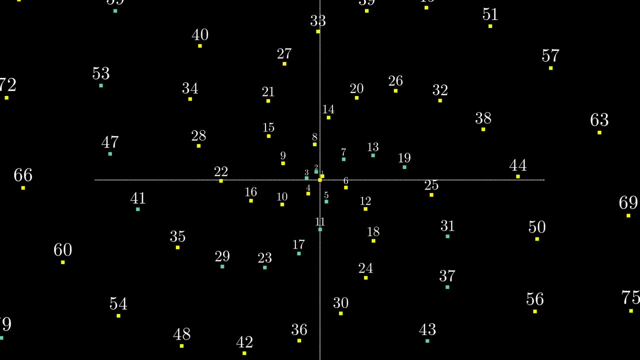 To kick things off, let's zoom back in a little bit smaller. Did you notice that as we were zooming out there were these six little spirals? This offers a good starting point to explain what's happening in the two larger patterns. 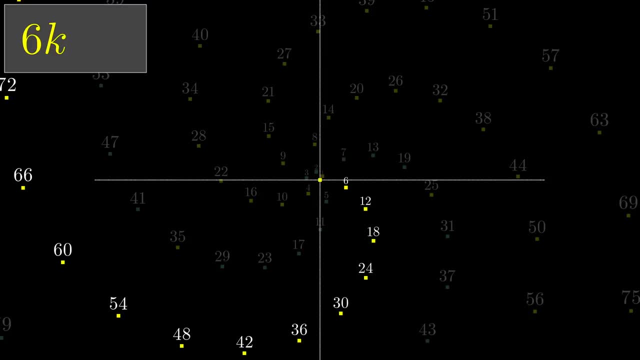 Notice how all the multiples of six form one arm of this spiral. Then the next one is every integer, that's one above a multiple of six, And then after that it includes all the numbers, The numbers two above a multiple of six, and so on. 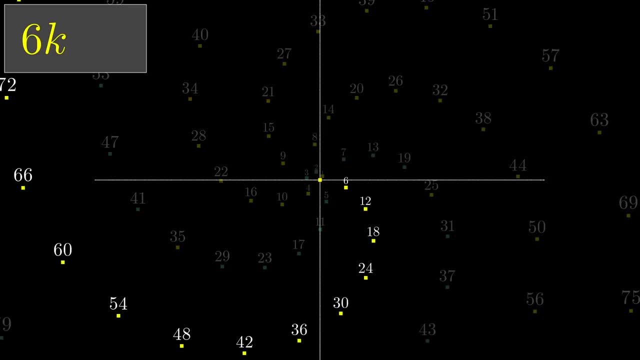 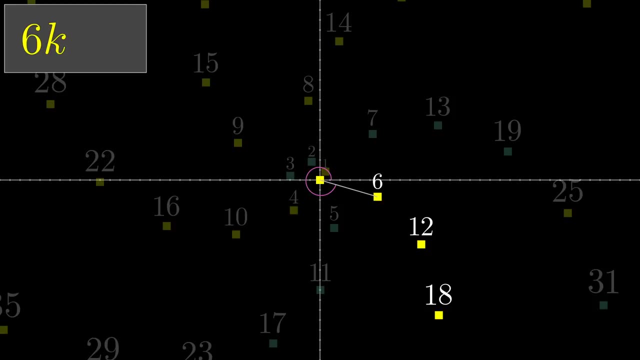 Why is that? Well, remember that each step forward in this sequence involves a turn of one radian. So when you count up by six, you've turned a total of six radians, which is a little bit less than two pi a full turn. 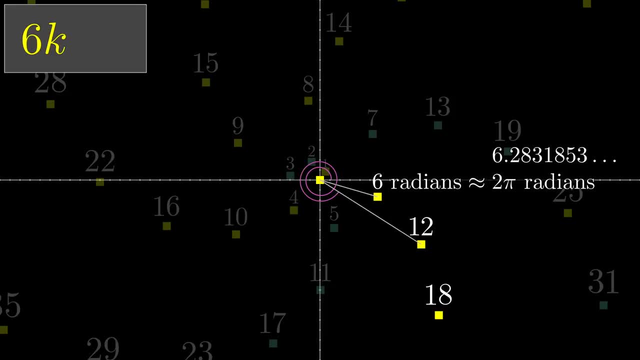 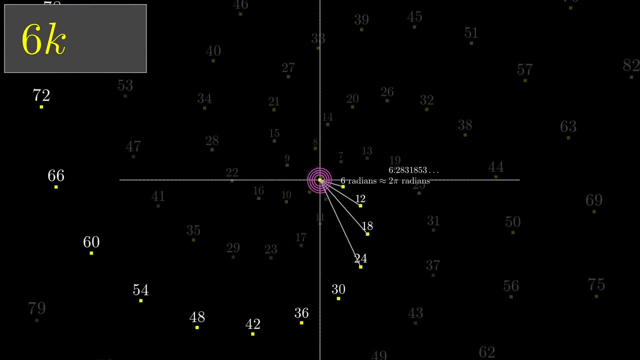 So every time you count up by six, you've almost made a full turn, It's just a little less: Another six steps, a slightly smaller angle, Six more steps smaller still, And so on, With this angle changing gently enough that it gives the illusion of a single curving. 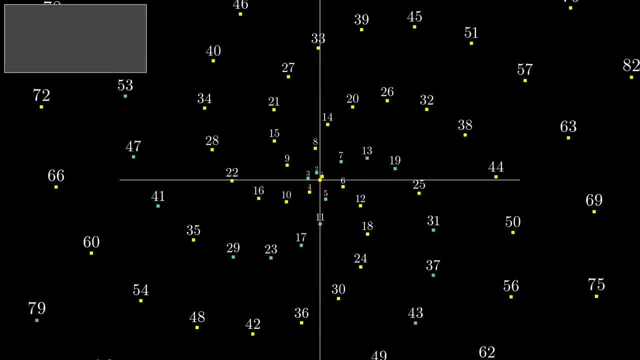 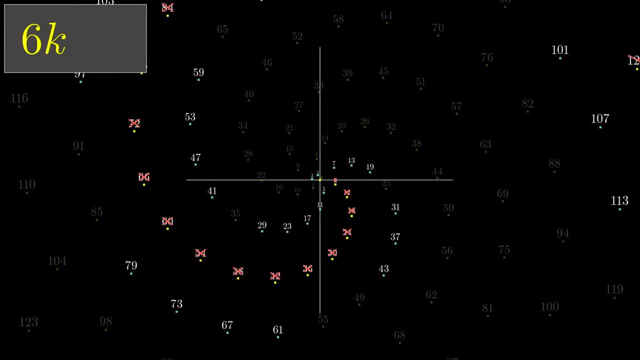 line. When you limit the view to prime numbers, all but two of these spiral arms will go away. And think about it. A prime number can't be a multiple of six, And it also can't be two above a multiple of six, unless it's two or four above a multiple. 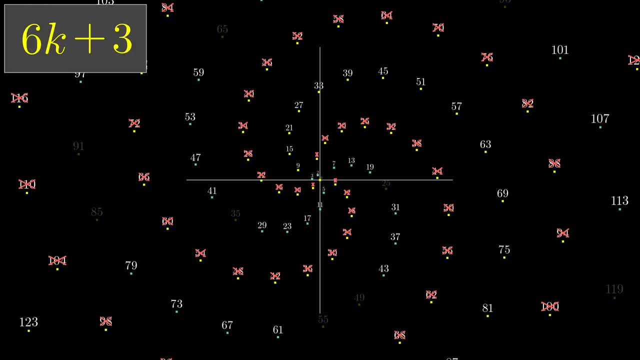 of six, since all of those are even numbers. It also can't be three above a multiple of six, unless it's the number three itself, since all of those are divisible by three. So at least in this smaller scale, nothing magical is going on. 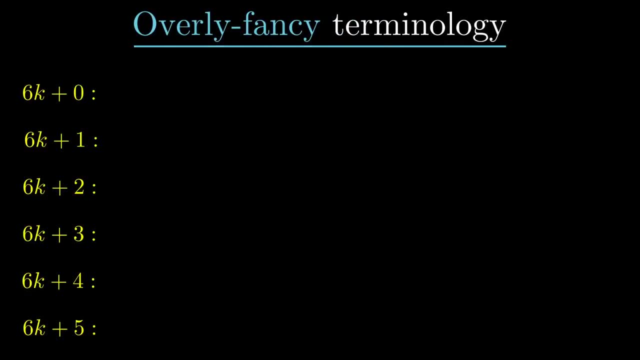 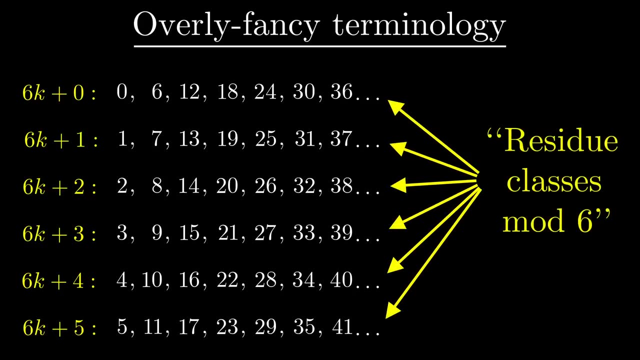 And while we're in this simpler context, let me introduce some terminology that mathematicians use. Each of these sequences where you're counting up by six is fancifully called a residue class mod six. The word residue here is just an overdramatic way of saying remainder, and mod means something. 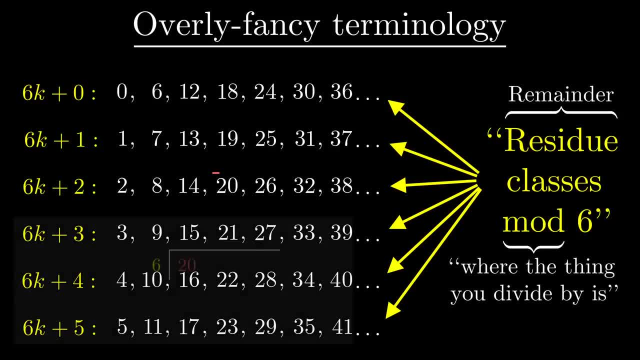 like where the thing you divide by is. For example, 6 goes into 20 three times. So if you add this up to six, it leaves a remainder of 10.. So my first thought is: what if I asked the question where the thing you divide by is? 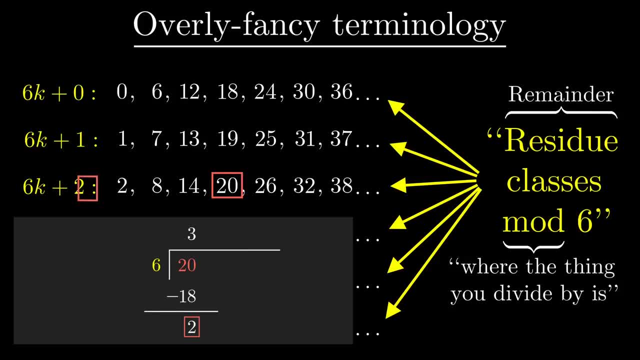 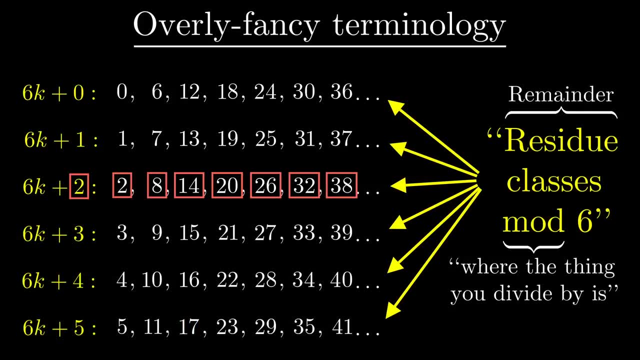 2.. So 20 has a residue of 2 mod 6.. Together with all the other numbers, leaving a remainder of 2 when the thing you divide by is 6, you have a full residue, class mod 6.. I know that sounds like the world's most pretentious way of saying everything. 2 above: 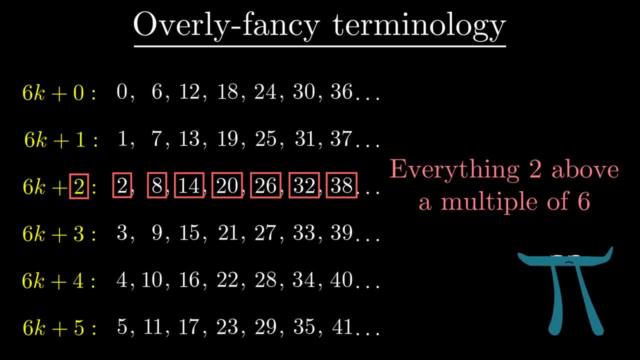 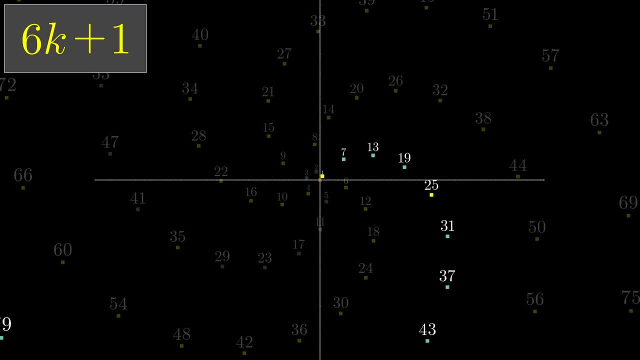 a multiple of 6,, but this is the standard jargon and it is actually handy to have some words for the idea. So, looking at our diagram, in the lingo each of these spiral arms corresponds to a residue class mod 6, and the reason we see them is that 6 is close to 2 pi turning 6 radians. 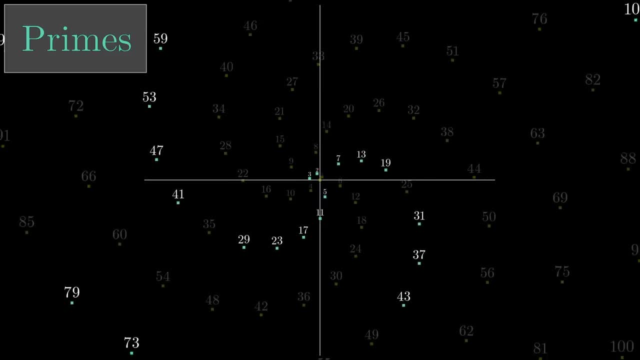 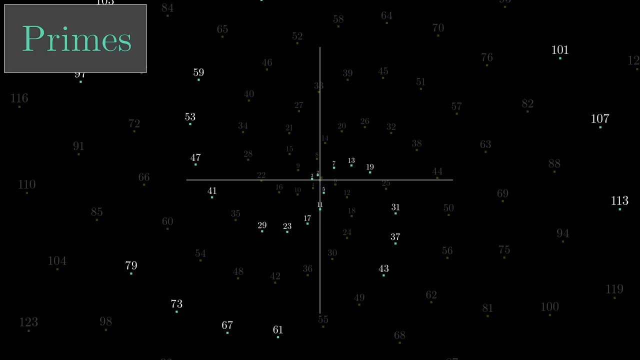 is almost a full turn, And the reason we see only 2 of them when filtering for primes is that all prime numbers are either 1 or 5 above a multiple of 6, with the exceptions of 2 and 3.. With all that as a warm up, let's think about the larger scale. 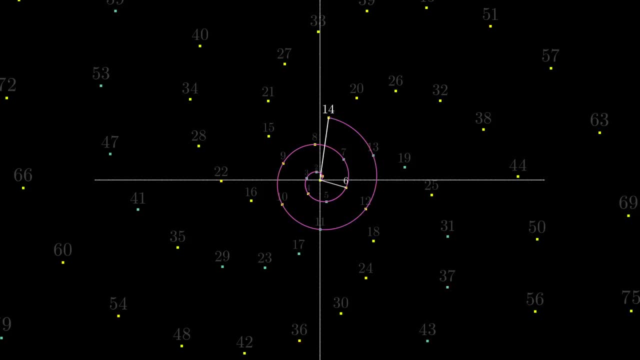 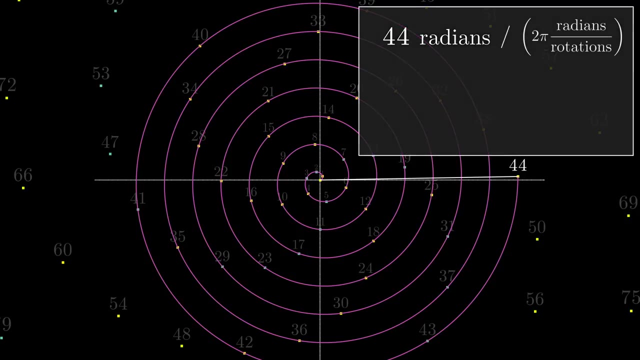 In the same way that 6 steps is close to a full turn, taking 44 steps is very close to a whole number of turns. Here let's compute it: There are 2 pi radians per rotation, right? So taking 44 steps, turning 44 radians, gives a total of 44 divided by 2 pi rotations, which. 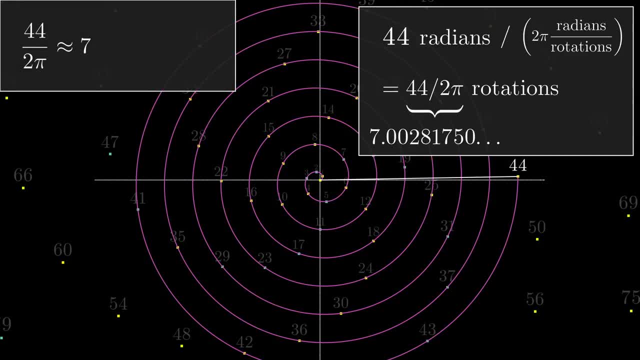 comes out to be just barely above 7 full turns. You could also write this by saying that 44 sevenths is a close approximation for 2 pi, which some of you may better recognize as the famous 22 sevenths approximation for pi. 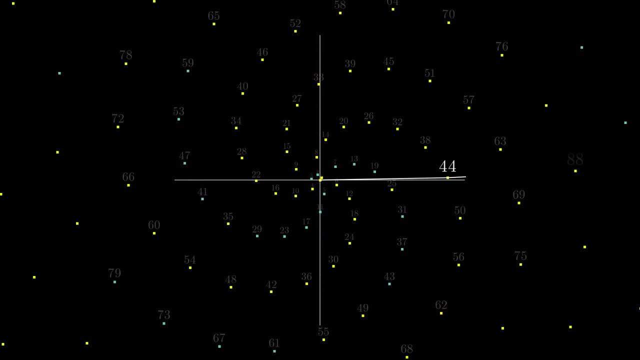 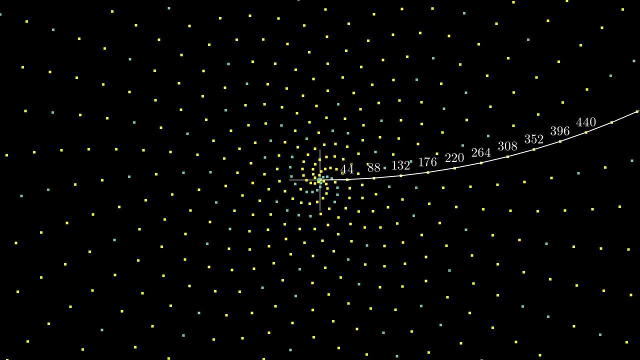 What this means is that when you count up by multiples of 44 in the diagram, each point has almost the same angle as the last one, just a little bit bigger. So as you continue on with more and more, we get this very gentle spiral as the angle. 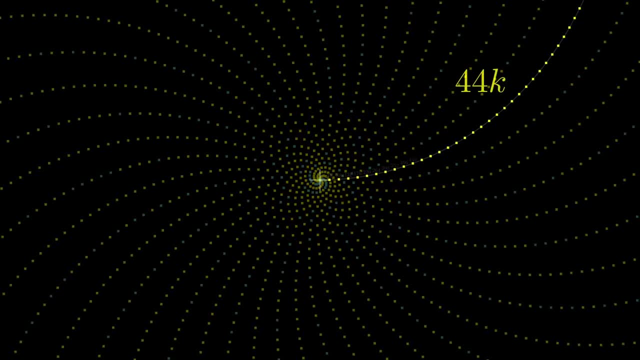 increases very slowly. Similarly, all the numbers 1 above a multiple of 44 make another spiral, but rotated one radian, counterclockwise. Same for everything: 2 above a multiple of 44, and so on, eventually filling out the 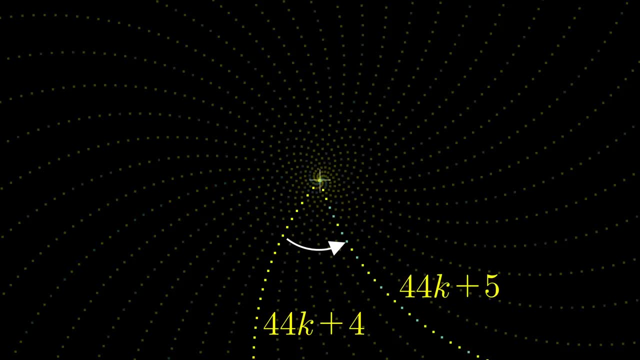 full diagram. To phrase it with our fancier language, each of these spiral arms shows a residue class, mod 44. And maybe now you can tell me what happens when we limit our view to prime numbers. Primes cannot be a multiple of 44, so that arm won't be visible. 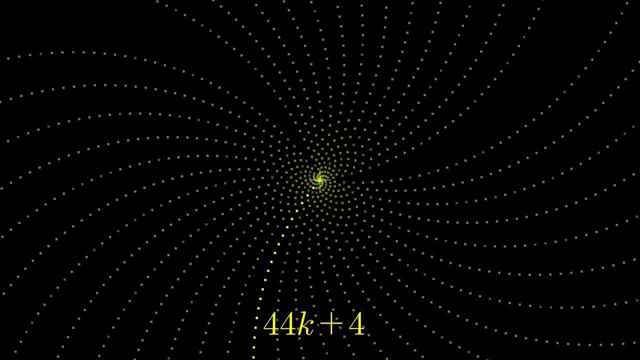 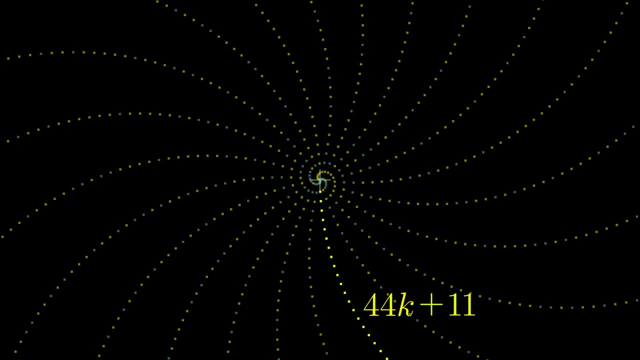 Nor can a prime be 2 above a multiple of 44, or 4 above and so on, since all those residue classes have nothing but even numbers. Likewise, Any multiples of 11 can't be prime, except for 11 itself. 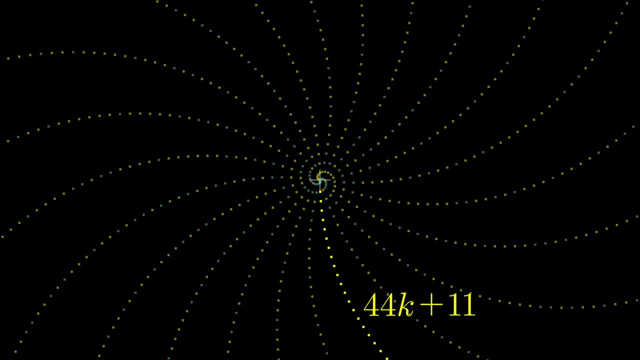 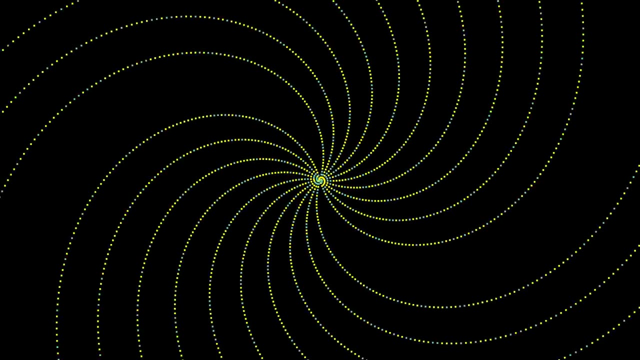 So the spiral of numbers 11 above a multiple of 44 won't be visible, and neither will the spiral of numbers 33 above a multiple of 44. This is what gives the picture, those milky-way-seeming gaps. Each spiral we're left with is a residue class that doesn't share any prime factors. 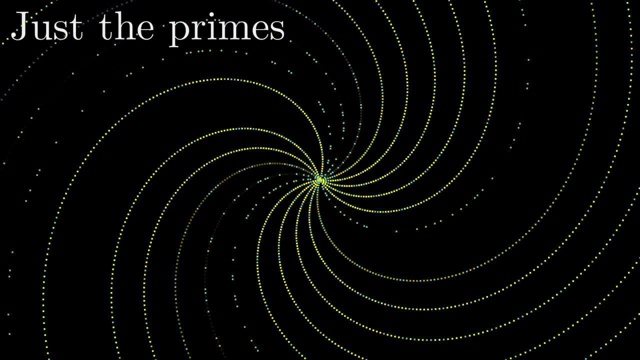 with 44., And within each one of those arms that we can't reject out of hand, the prime numbers seem to be sort of randomly distributed, And that's a fact that I'd like you to check out in the next video. Thanks for watching. 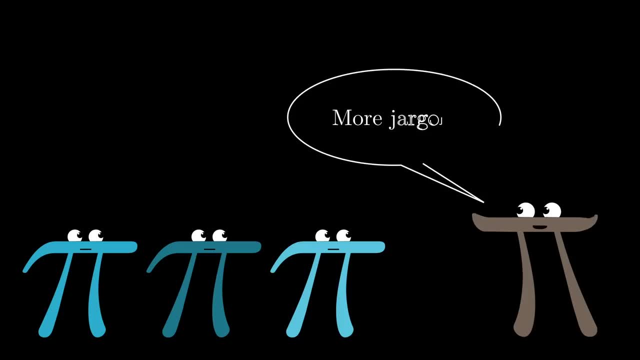 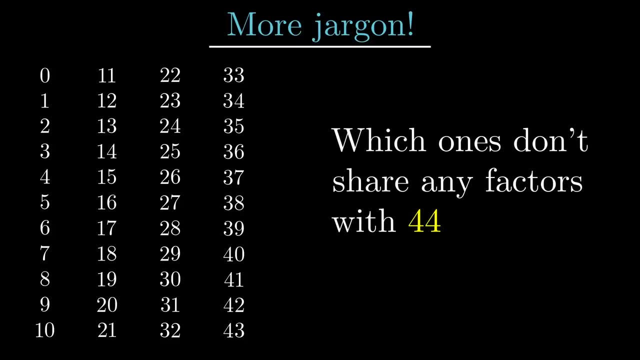 Tuck away. we'll return to it later. This is another good chance to inject some of the jargon that mathematicians use. What we care about right here are all the numbers between 0 and 43 that don't share a prime factor with 44, right. The ones that aren't even, and they also aren't divisible by 11.. When two numbers don't share any factors like this, we call them relatively prime or also co-prime. In this example, you could count that there are 20 different numbers between 1 and 44,. 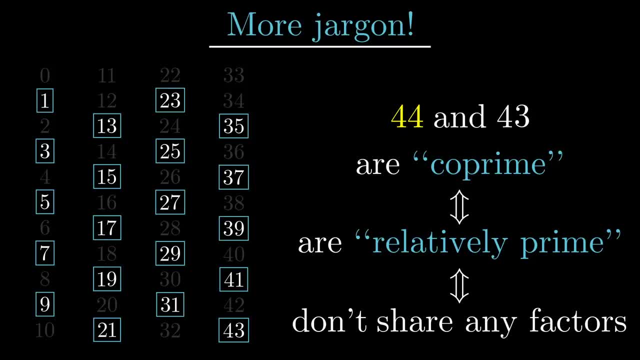 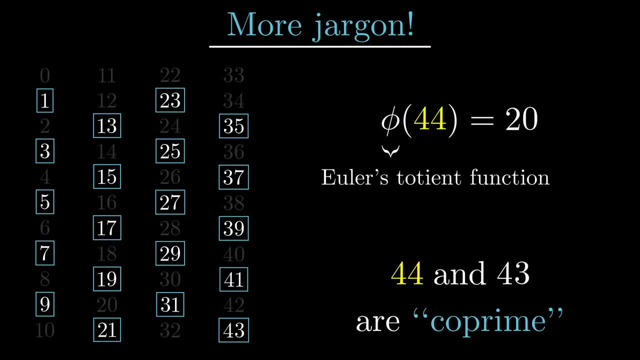 and this is a fact that a number theorist would compactly write by saying: phi of 44 equals 20, where the Greek letter phi here refers to Euler's totient function- yet another needlessly fancy word- which is defined to be the number of integers from 1 up to n, which 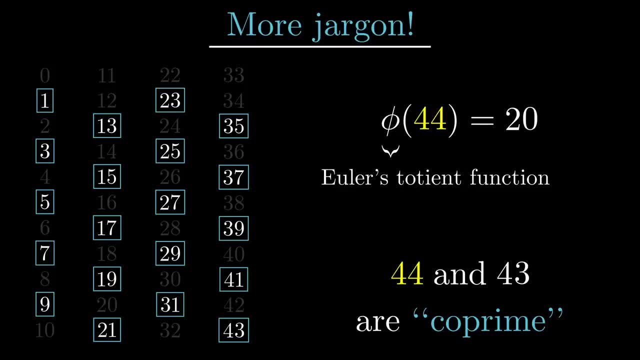 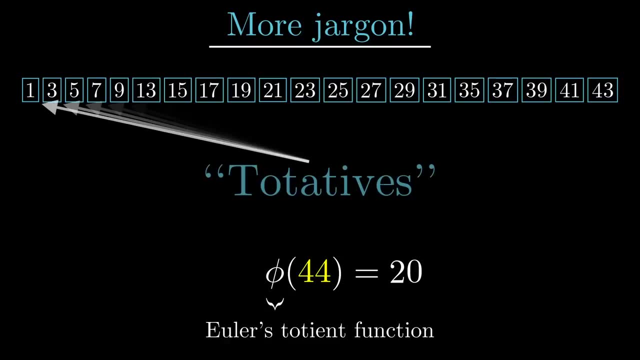 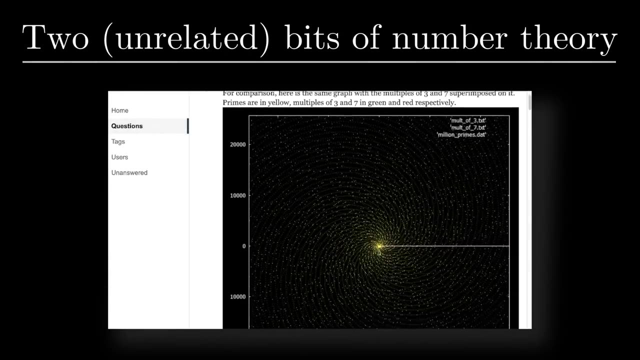 are co-prime to n. It comes up enough that it's handy to have compact notation More obscurely, and I had never heard this before, but I find it too delightful not to tell It's the totative of n. Back to the main thread. in short, what the user on math exchange was seeing are two unrelated. 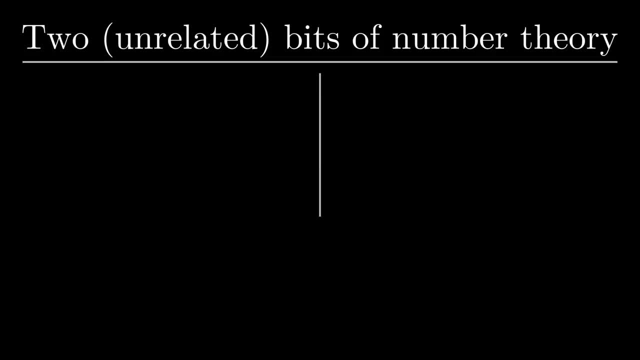 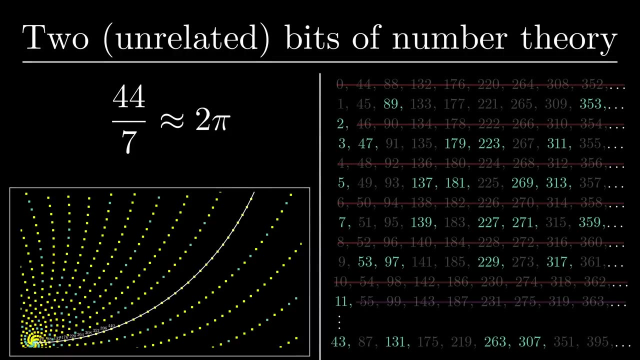 pieces of number theory but illustrated in one drawing. The first is that 44 sevenths is a very close rational approximation for 2 pi, which results in the residue classes mod 44 being cleanly separated out. The second is that many of these residue classes contain zero prime numbers or sometimes just 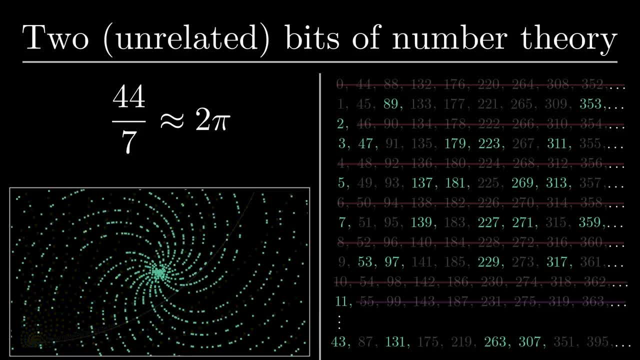 one, so they won't show up. But on the other hand, primes do show up. Primes do show up plentifully enough in all 20 of the other residue classes that it makes these spiral arms visible, And at this point maybe you can predict what's going on at the larger scale. 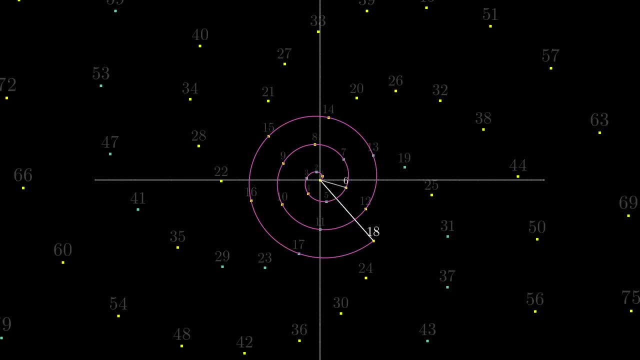 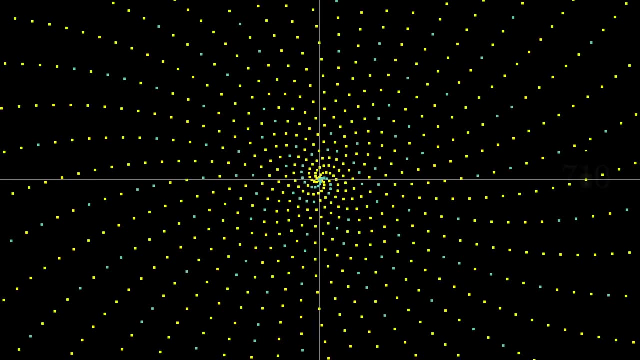 Just as 6 radians is vaguely close to a full turn and 44 radians is quite close to 7 full turns, it just so happens that 710 radians is extremely close to a whole number of full turns Visually. you can see this by the fact that the point ends up almost exactly on the x-axis. 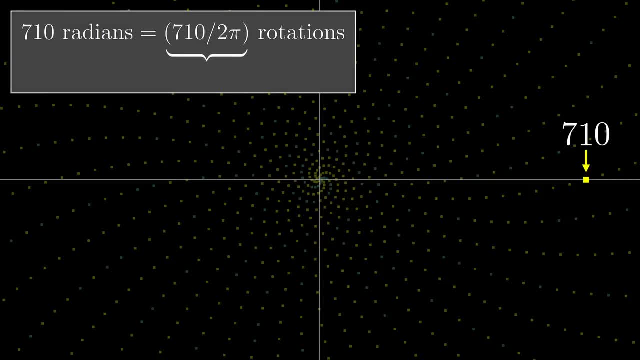 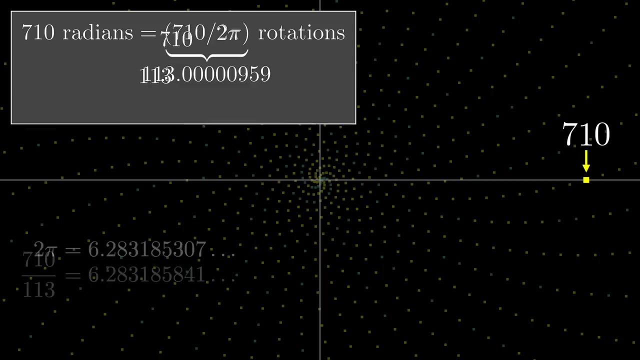 but it's more compelling: analytically, 710 radians is 710 divided by 2 pi rotations, which works out to be 113.000095.. Some of you may have seen this in another form. It's saying that 710, one hundred thirteenths, is a close approximation for 2 pi, which is 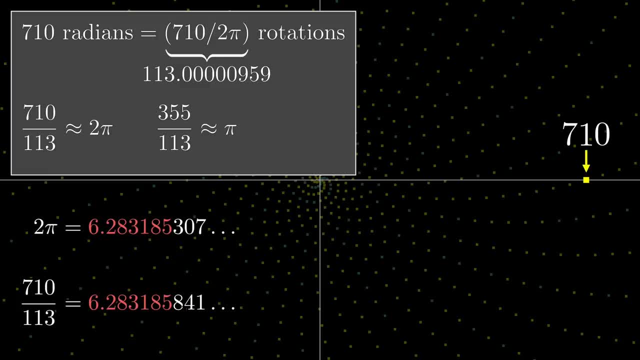 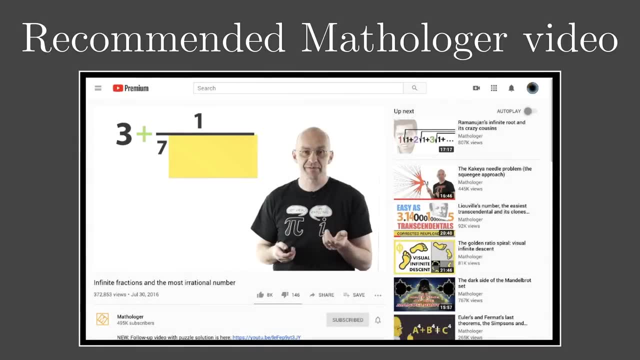 more commonly seen in saying that 355 over 113 is a very good approximation for pi. Now, if you want to understand this, you can do this. Let's do it If you want to understand where these rational approximations are coming from and what it. 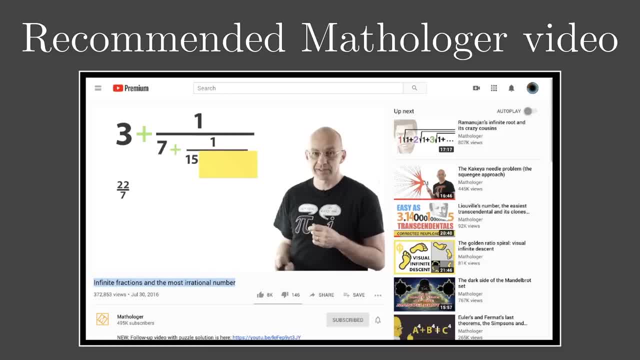 means for one like this to be unusually good, like way better than you would get for phi or e or square root of 2 or other famous irrationals. I highly recommend taking a look at this great Mathologer video. For our storyline, though, it means that when you move forward by steps of 710, the angle 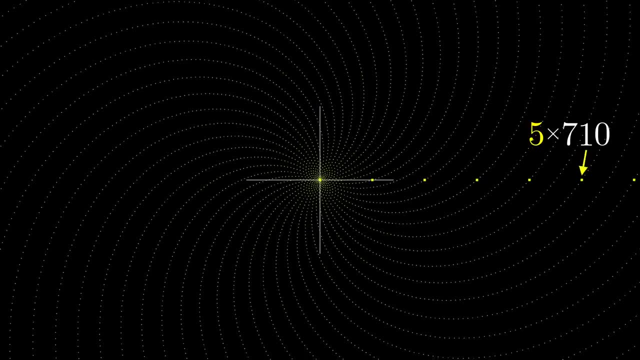 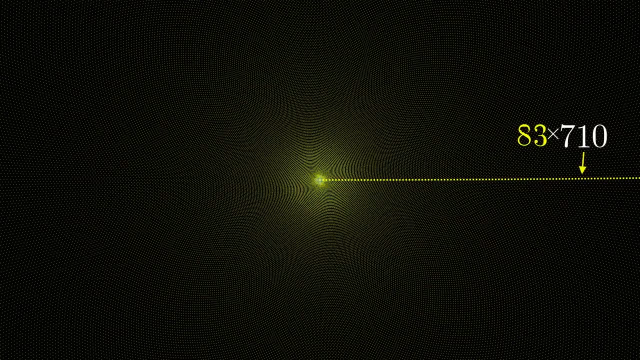 of each new point is almost exactly the same as the last one, just microscopically bigger. Even very far out, One of these sequences looks like a straight line, And of course the other residue classes, mod 710, also form these nearly straight lines. 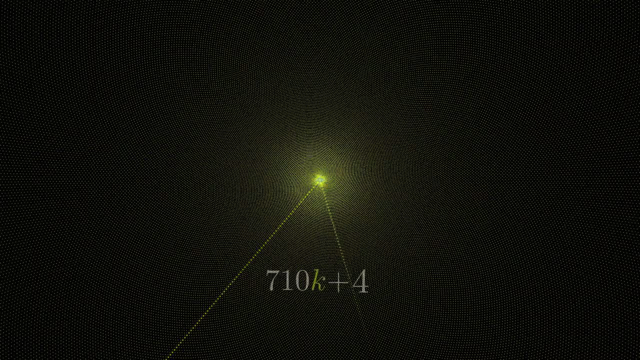 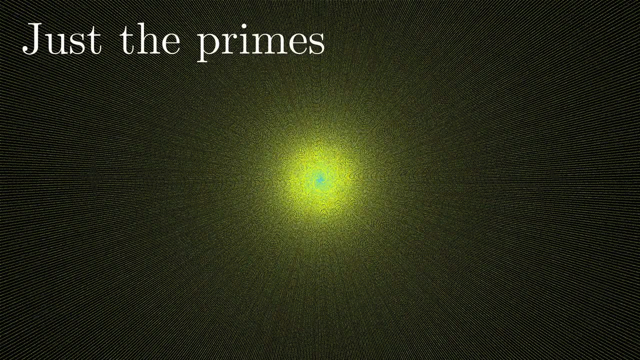 710 is a big number, though, so when all of them are on screen and there's only so many pixels on the screen, it's a little hard to make them out. So in this case it's actually easier to see when we limit the view to primes, where you 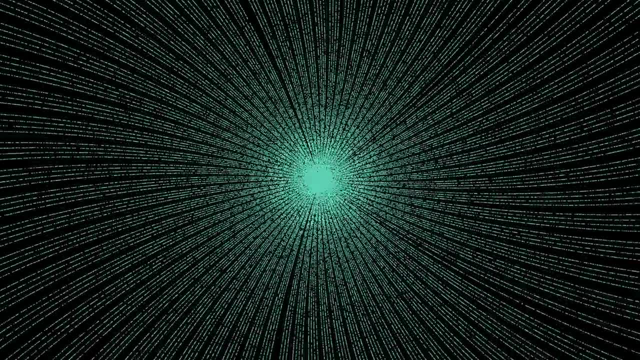 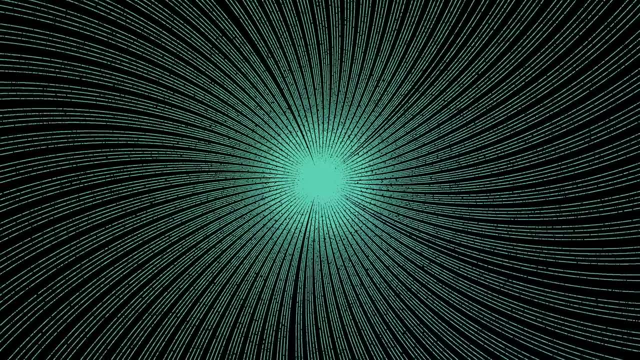 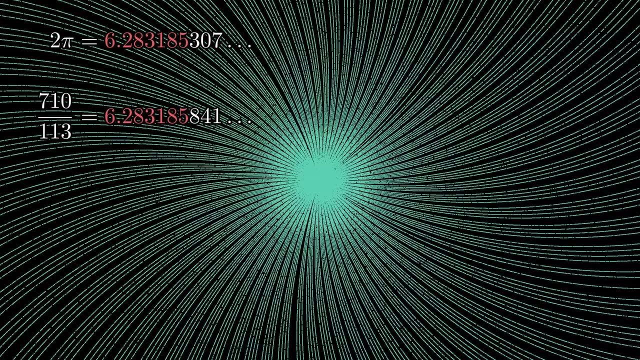 don't see many of those residue classes In reality. with a little further zooming you can see that there actually is a very gentle spiral to these. But the fact that it takes so long to become prominent is a wonderful illustration- maybe the best illustration I've ever seen- for just how good an approximation this is for. 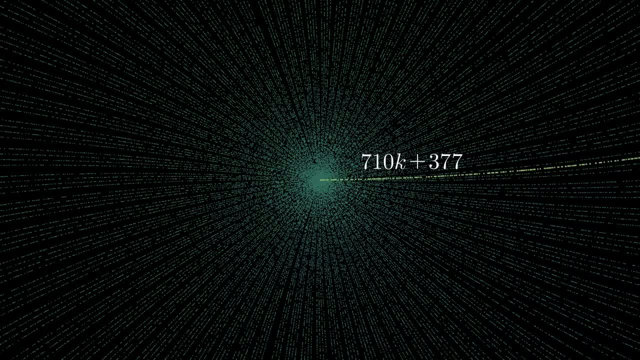 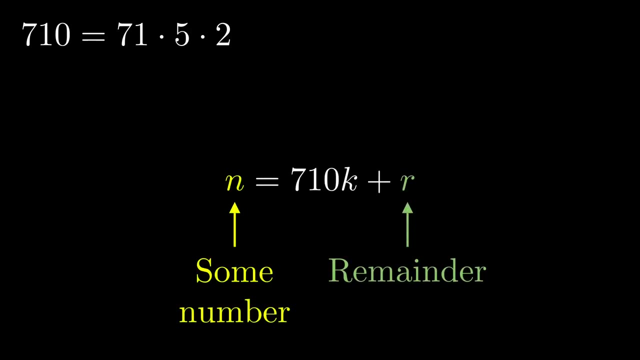 2pi, Tying up the remaining loose thread here. if you want to understand what happens when you filter for primes, it's entirely analogous to what we did before. The factors of 710 are 71,, 5, and 2, so if the remainder or residue is divisible by, 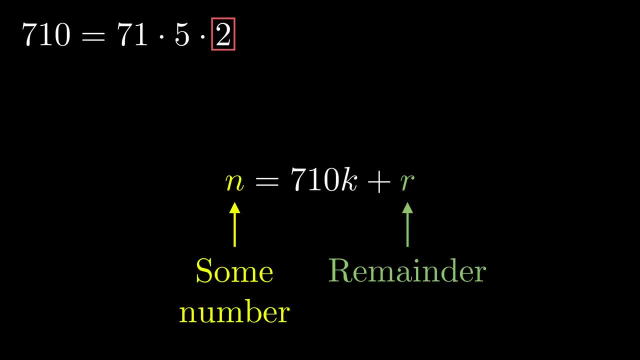 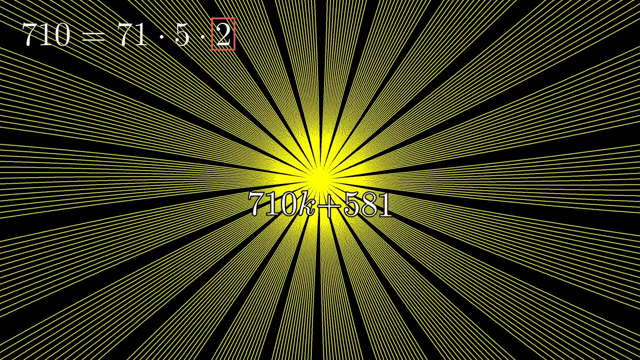 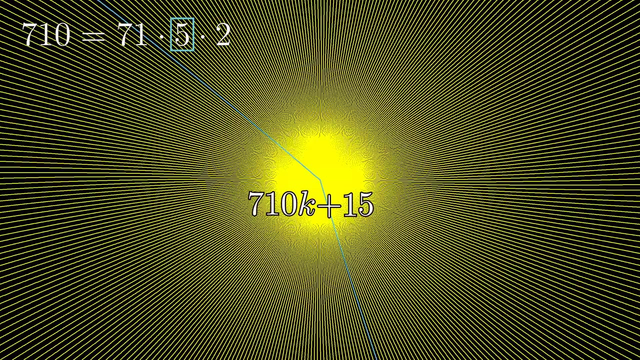 any of those, then so is the number. When you pull up all of the residue classes with odd numbers, it looks like every other ray in the otherwise quite crowded picture. And then of those that remain, these are the ones that are divisible by 5, which are nice. 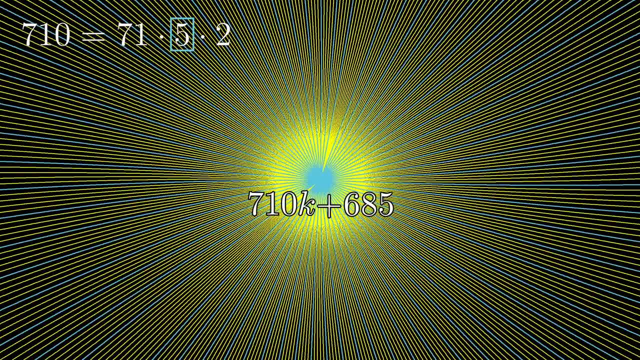 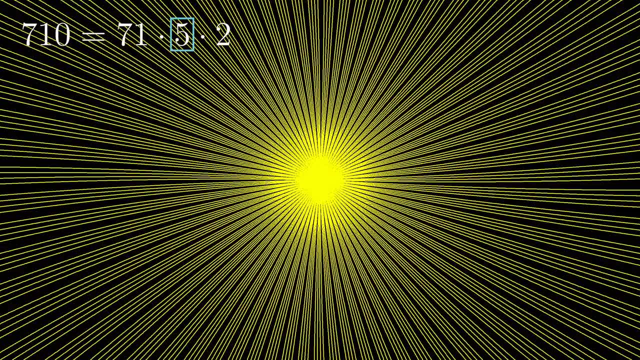 and evenly spaced at every 5th line. Notice the fact that prime numbers never show up in any of these is what explains the pattern of the lines we saw at the beginning coming in front of us. We can see that these lines are divisible by 5.. 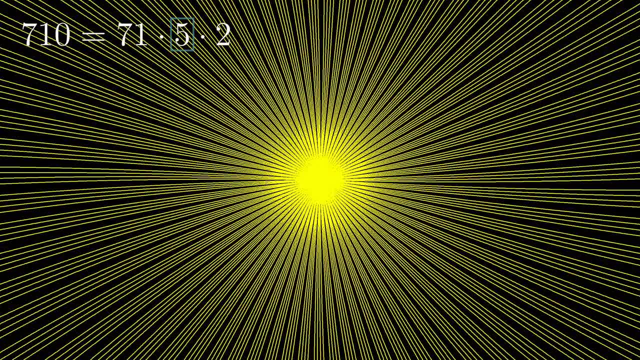 And, moreover, of those remaining, these 4 residue classes are the ones that are divisible by 71, so the primes aren't going to show up there, And that's what explains why the clumps of 4 we saw occasionally have a missing tooth. 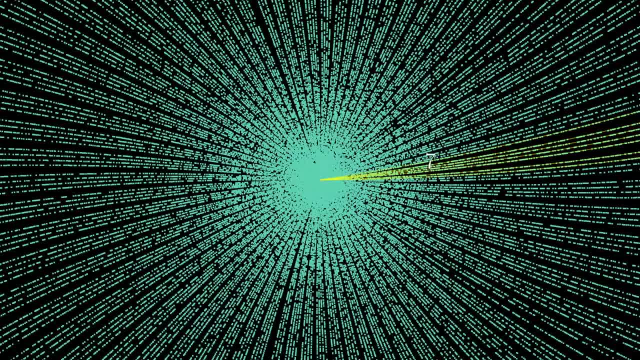 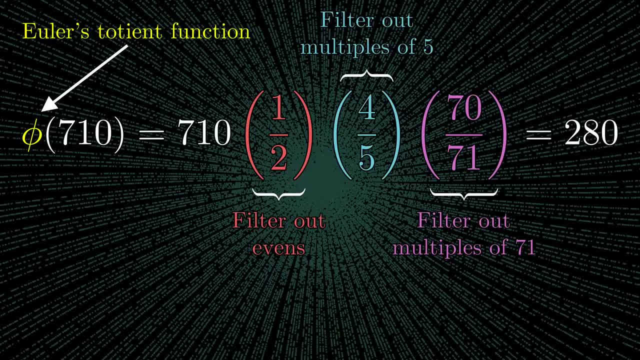 in your comb. And if you were wondering where that number 280 came from, it comes from counting how many of the numbers from 1 up to 710 don't share any prime factors with 710. These are the ones we can't rule out. 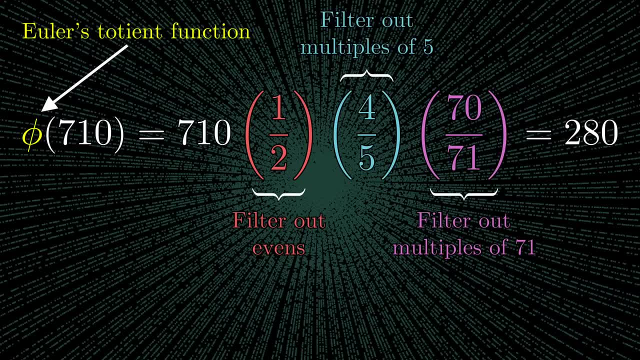 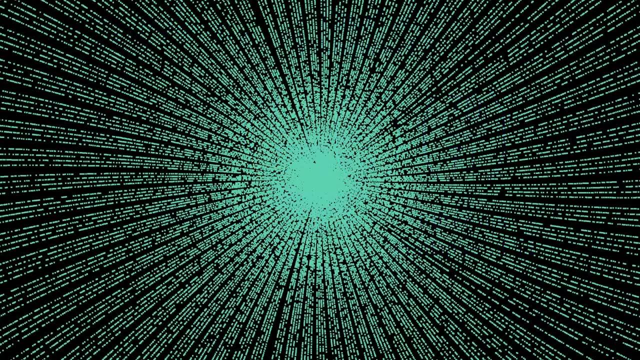 We can't rule out for including primes based on some obvious divisibility consideration. This of course doesn't guarantee that any particular one will contain prime numbers, but at least empirically, when you look at this picture, it actually seems like the primes are pretty evenly distributed among the remaining classes, wouldn't you agree? 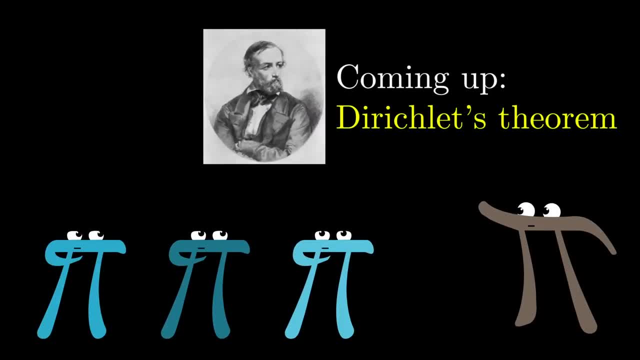 This last point is actually the most interesting observation of the whole deal. It relates to a pretty deep fact in number theory known as Dirichlet's Theorem. To tell you the truth, it's a pretty deep fact. It's called Dirichlet's Theorem. 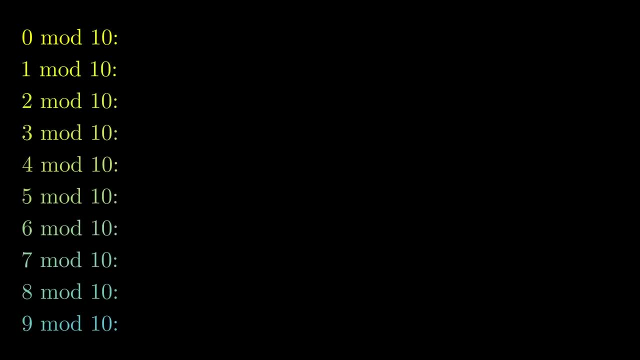 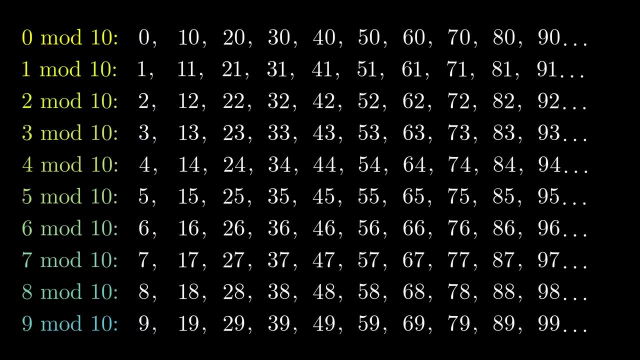 If we take a simpler example than residue classes, mod 7, 10, think of those mod 10.. Because we write numbers in base 10, this is the same thing as grouping numbers together by what their last digit is. Everything whose last digit is 0 is a residue class. everything whose last digit is 1 is. 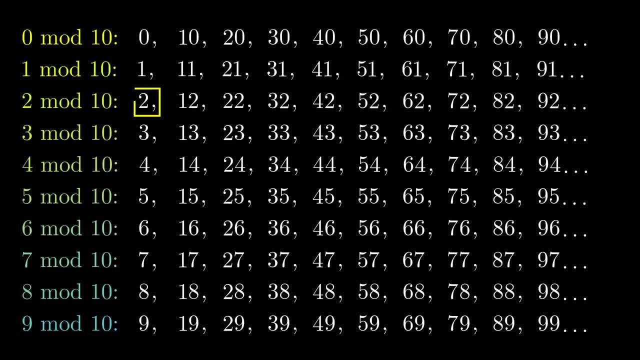 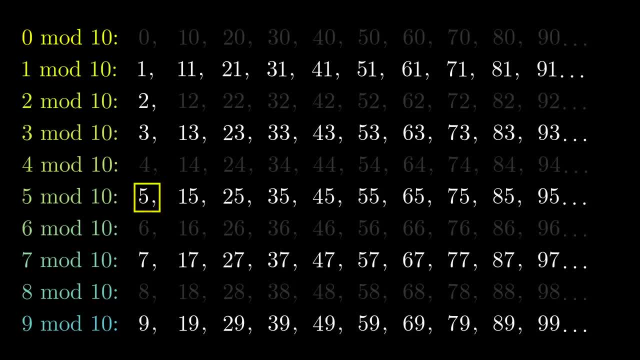 another residue class, and so on. Other than 2, prime numbers can't have an even number as their last digit, since that means they're even, And likewise any prime bigger than 5 can't end in a 5.. There's nothing surprising there. that's one of the first facts you observe when you 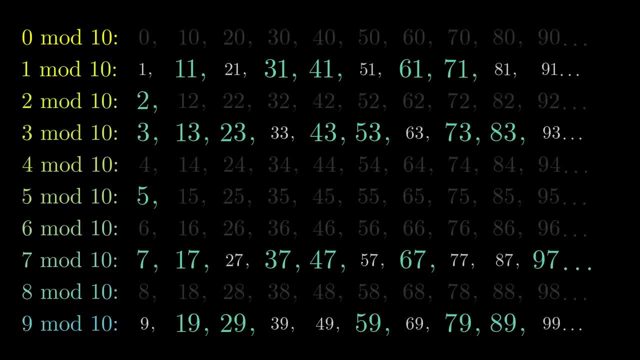 learn about prime numbers. Anything bigger than 5 has to end in either a 1,, a 3,, a 7, or a 9.. A much more nuanced question, though, is how exactly these primes are divvied up among those. 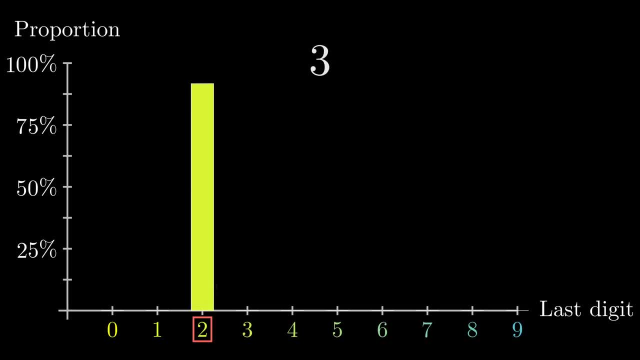 remaining 4 groups. Here let's make a quick histogram counting through each prime number where the bars are going to show what proportion of the primes we've seen so far have a given last digit. So in particular the 2 and 5 slots should go down to 0 over time. 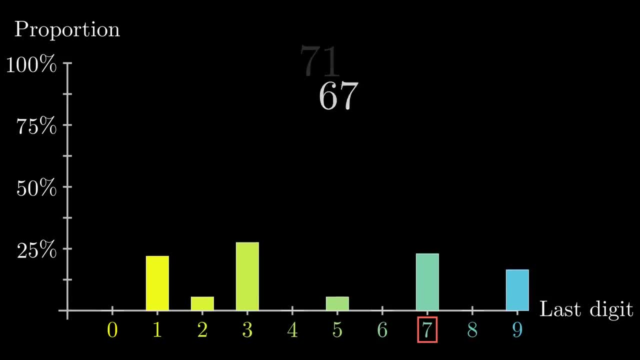 What would you predict is going to happen as we move forward? Well, as we get a lot of them, it seems like a pretty even spread between these 4 classes, about 25% each, And probably that's what you would expect, after all. why would prime numbers show some? 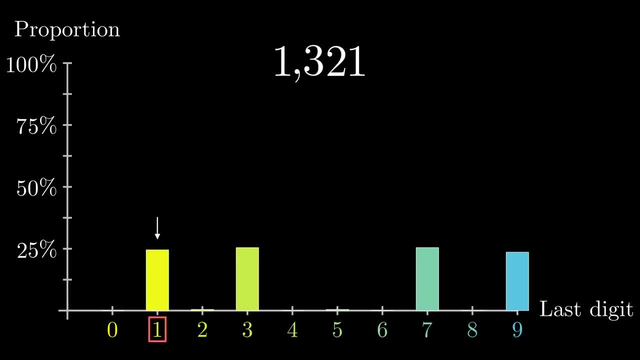 sort of preference for one last digit over another. But primes aren't random. they are a definite sequence and they show patterns in other ways, and it's highly non-obvious how you would prove something like this Or, for that matter, how do you rigorously phrase what it is that you want to prove? 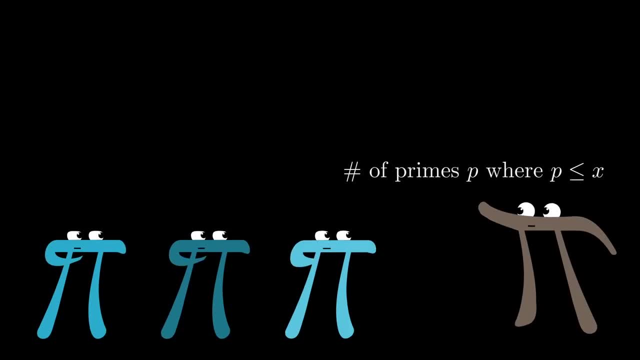 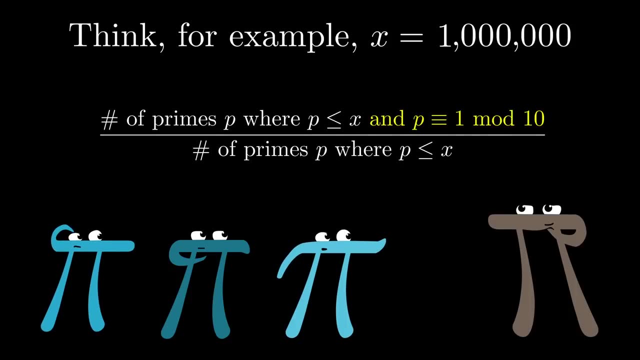 A mathematician might go about it something like this: If you look at all the prime numbers- less than some big number, x- and you consider what fraction of them are- say 1 above a multiple of 10, that fraction should approach 1. fourth, 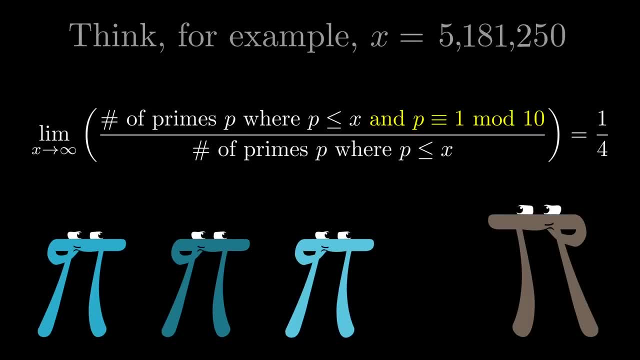 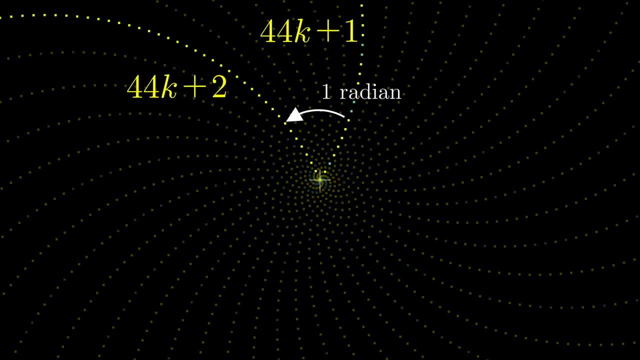 as x approaches infinity, And likewise for all of the other allowable residue classes, like 3 and 7 and 9.. Of course, there's nothing special about 10,. a similar fact should hold for any other number, Considering our old friends the residue classes mod44,, for example. let's make a similar. 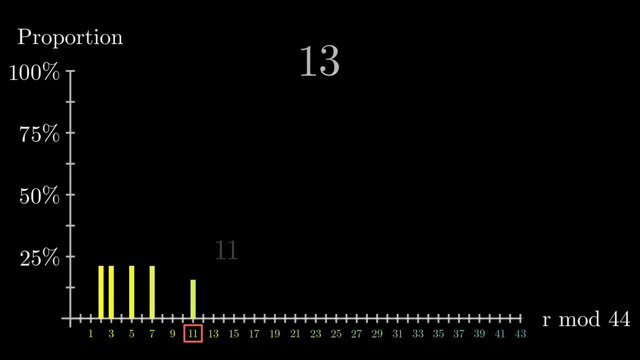 histogram showing what proportion of the primes show up in each one of these. Again, as time goes on, we see an even spread between the 20 different allowable residue classes. This is relative in terms of each spiral arm from our diagram having about the same number. 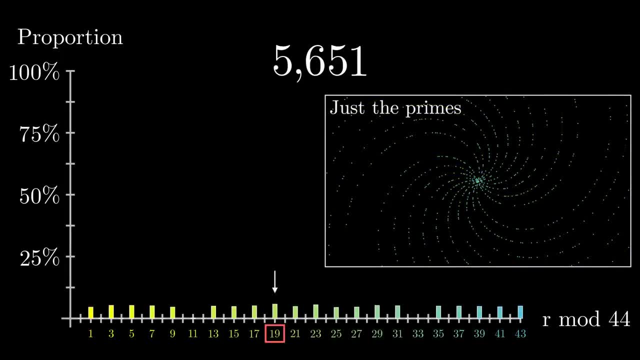 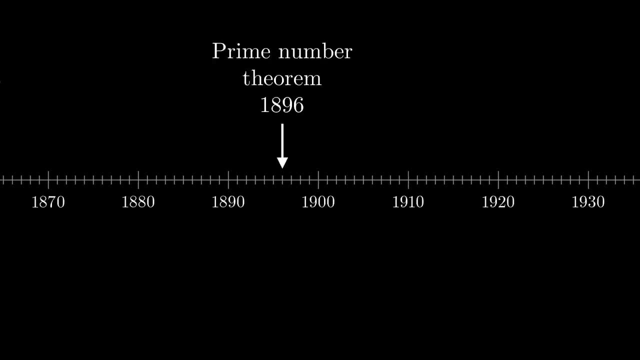 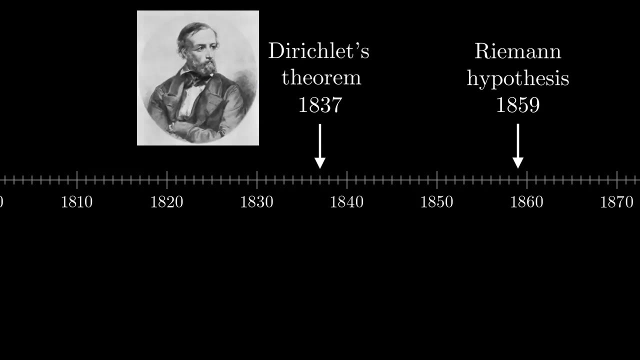 of primes as each of the others. Maybe that's what you'd expect, but this is a shockingly hard fact to prove. The first man who cracked this puzzle was Dirichlet in 1837, and it forms one of the crowning jewels at the foundation of modern analytic number theory. 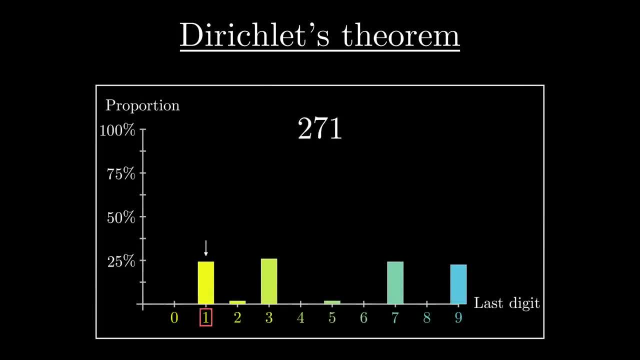 Histograms like these ones give a pretty good illustration of what the theorem is actually saying. Nevertheless, you might find it enlightening to see how it might be written. in the first case, It's essentially what we just saw for 10,, but more general. 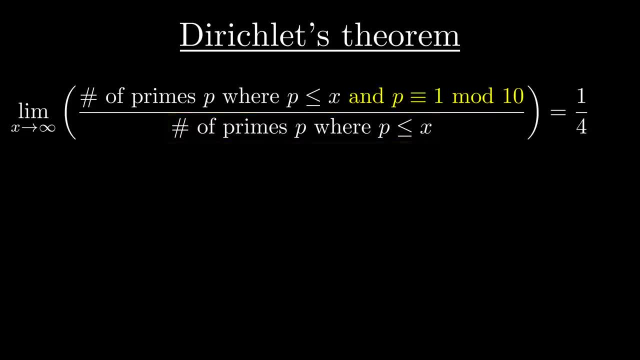 Again, you look at all of the primes up to some bound x, but instead of asking for what proportion of them have a residue of, say, 1 mod 10, you ask what proportion have a residue of r mod n, where n is any number and r is anything that's co-primed to n. 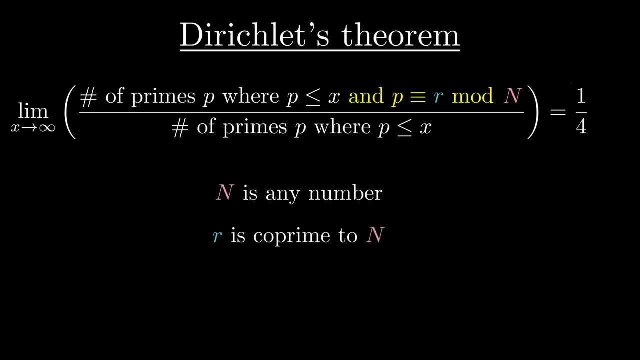 Remember that means it doesn't share any factors with n bigger than 1.. So what's the answer? Instead of approaching 1, fourth, as x goes to infinity, that proportion goes to 1 divided by phi of n, where phi is that special function I mentioned earlier that gives the number. 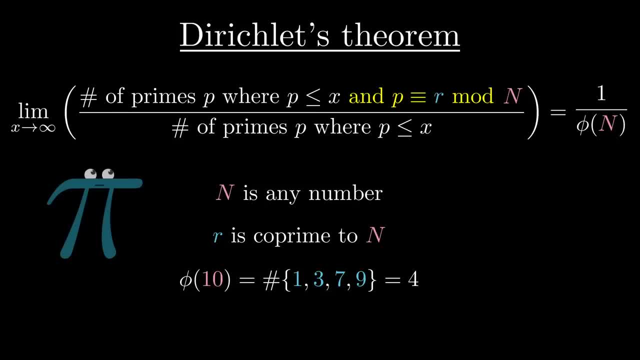 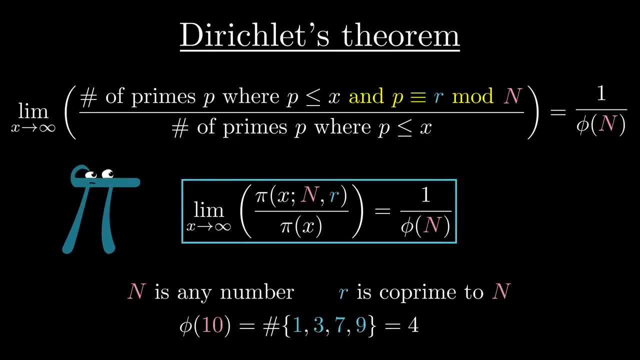 of possible residues co-primed to n. And in case this is too clear for the reader, you might see it buried in more notation. where this denominator and the numerator are both written with a special prime-counting function, The convention, rather confusingly, is to use the symbol pi for this function even. 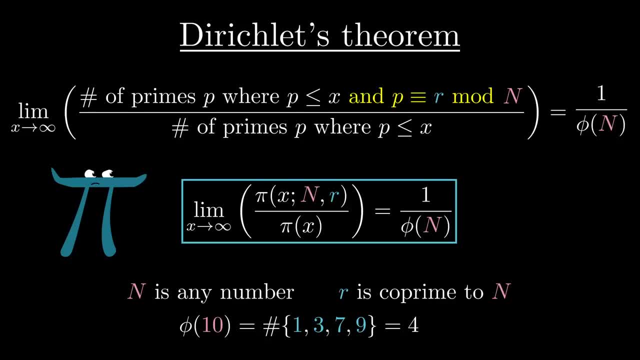 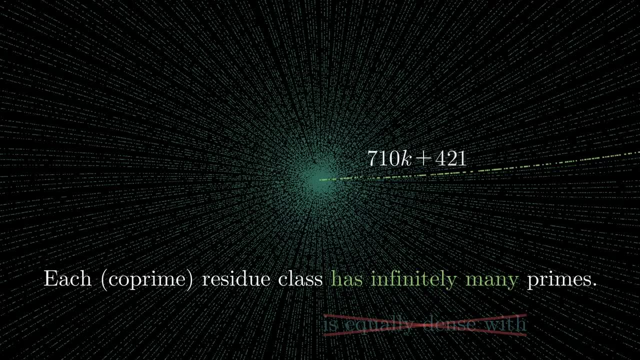 though it's totally unrelated to the number pi. In some contexts, when people refer to Dirichlet's theorem, they refer to a much more modest statement, which is simply that each of these residue classes that might have infinitely many primes does have infinitely many. 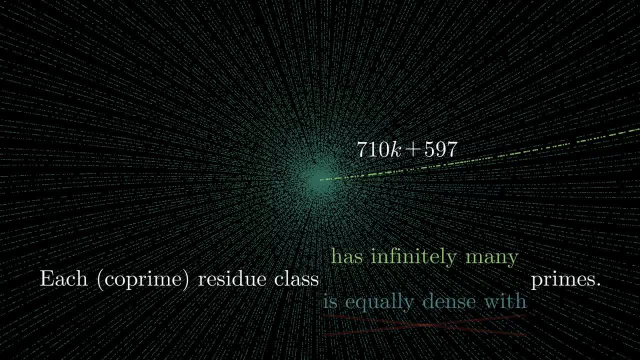 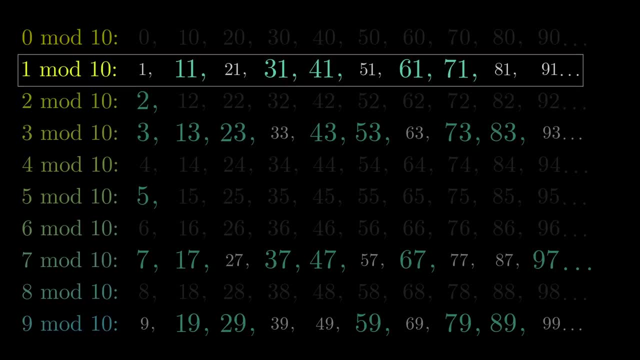 In order to prove this, what Dirichlet did was show that the primes are just as dense in any one of these residue classes as in any other. For example, imagine someone asks you to prove that there are infinitely many primes ending in the number 1, and the way you do it is by showing that a quarter of all the primes 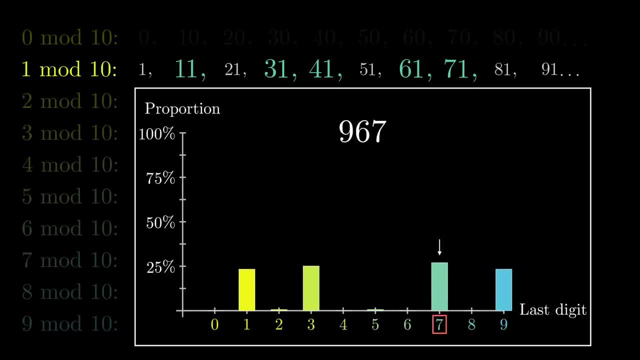 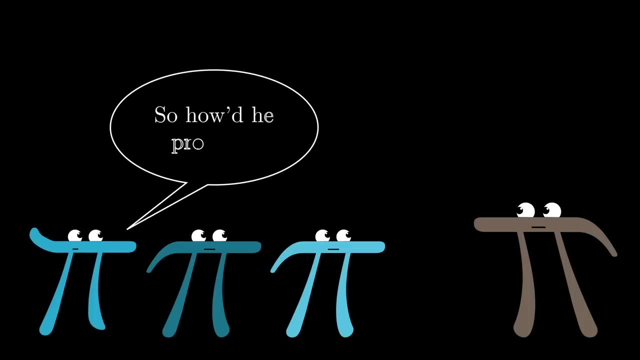 end in a 1.. Together with the fact that there are infinitely many primes which we've known since Euclid, this gives a stronger statement and a much more interesting one. Now the proof: well, it's way more involved than would be reasonable to show here. 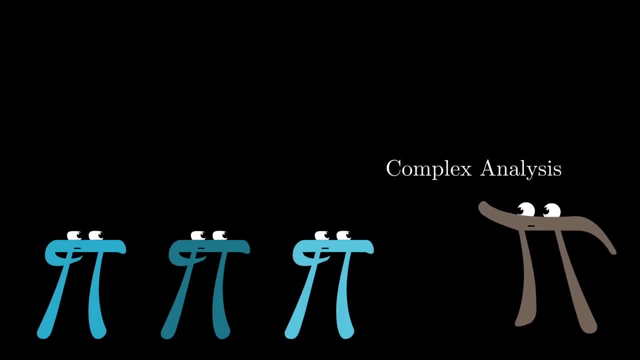 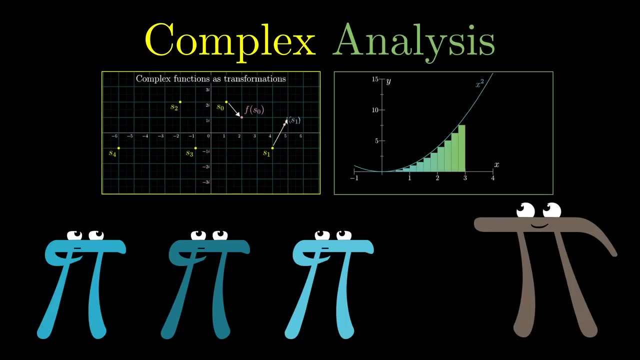 One interesting fact worth mentioning is that it relies heavily on complex analysis, which is the study of doing calculus with functions whose inputs and outputs are complex numbers. Now that might seem weird. right, I mean prime numbers seem wholly unrelated to the continuous world of calculus, much less when complex numbers end up in the mix. 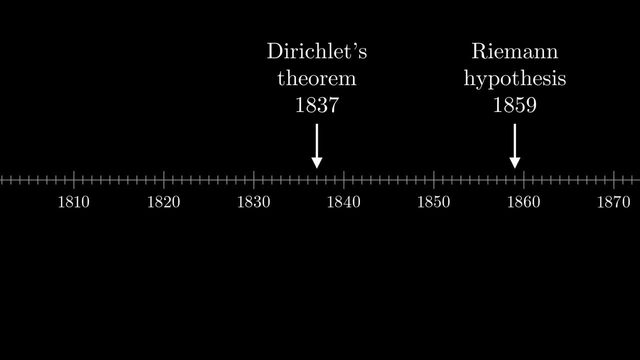 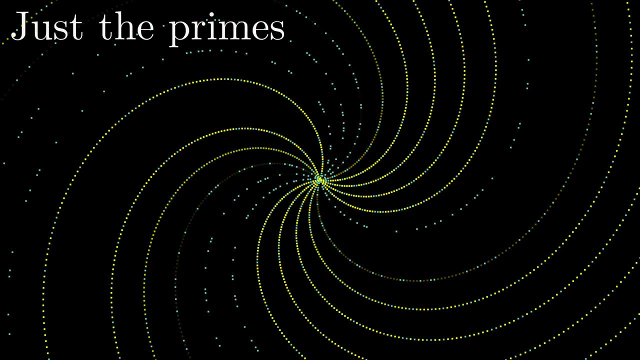 But since the early 19th century this is absolutely par for the course when it comes to understanding how primes are distributed. And this isn't just antiquated technology either. understanding the distribution of primes in residue classes like this continues to be relevant in modern research too. 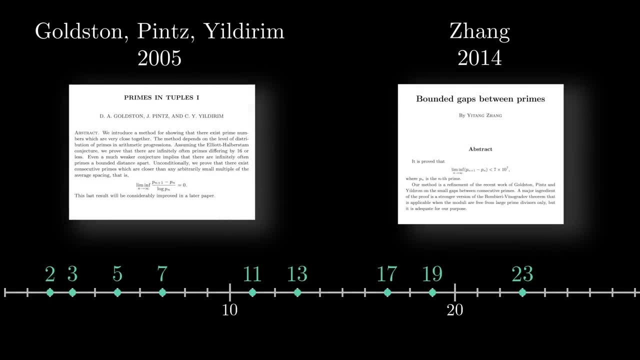 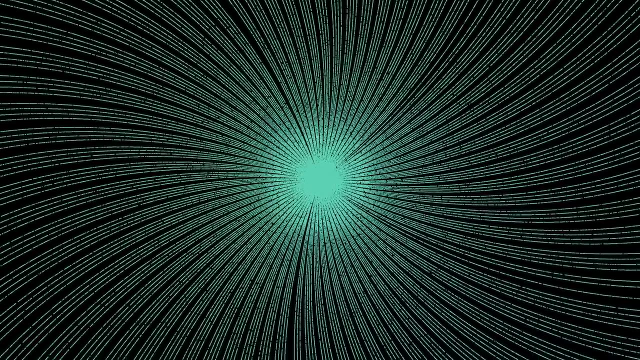 Some of the recent breakthroughs on small gaps between primes, edging towards that ever-elusive twin prime conjecture, have their basis in understanding how primes split up among these kinds of residue classes. Okay, looking back over the puzzle, I want to emphasize something. 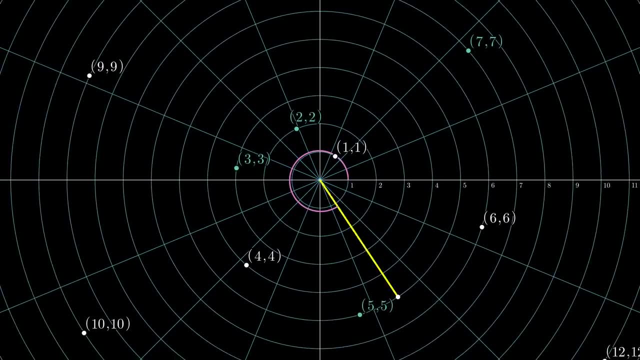 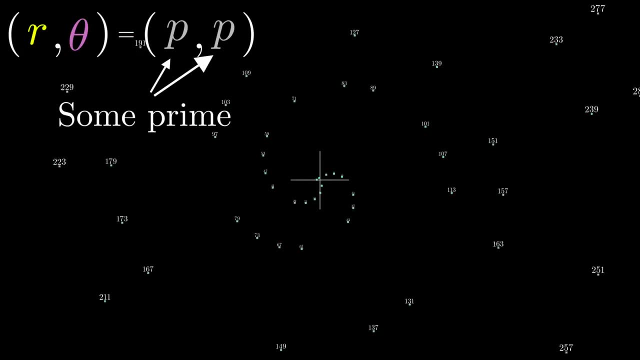 The original bit of data visualization whimsy that led to these patterns. well, it doesn't matter, no one cares. there's nothing special about plotting in polar coordinates, and most of the initial mystery in these spirals resulted from the artifacts that come from. 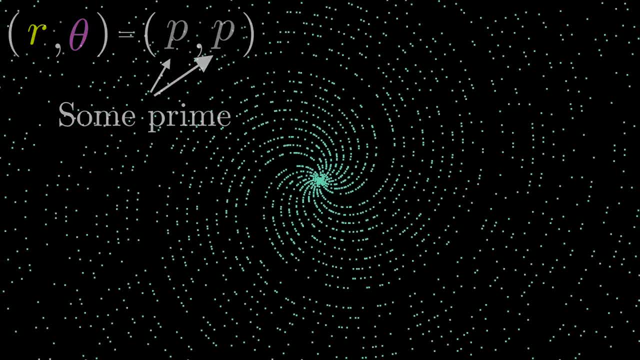 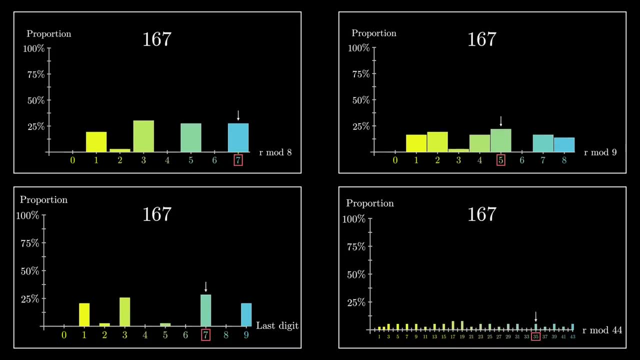 dealing with integer number of radians, which is kind of weird, But on the other hand, It's clearly worth it if the end result is a line of questions that leads you to something like Dirichlet's theorem, which is important, especially if it inspires you to learn enough.